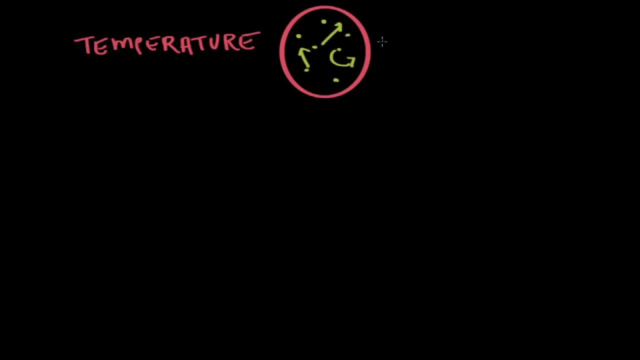 All of these little particles are moving And the energy of motion is called the kinetic energy. So all of these moving particles have kinetic energy. And so the faster those little particles are moving, the greater their kinetic energy. And if each of those little particles 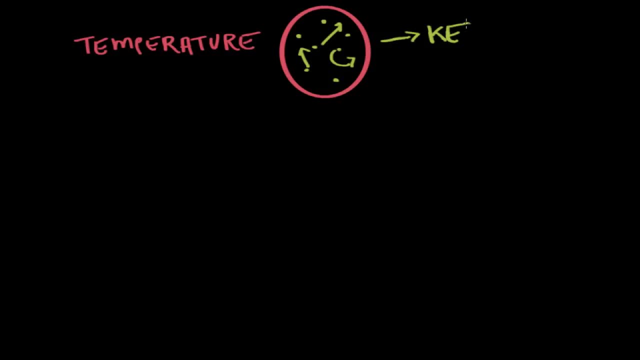 in the system has greater kinetic energy. that means the system as a whole has a larger amount of total energy And we would say that it has a greater temperature Because, again, temperature is a measure of the average kinetic energy of those particles And because knowing the amount of energy in a system can be really 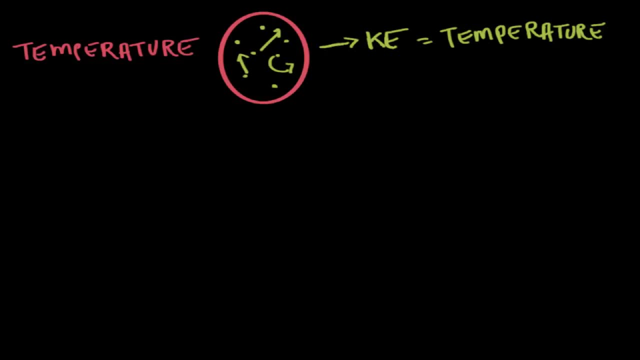 useful. in chemistry and in physics, we've developed temperature scales to help us quantify or measure the amount of this value, this value of energy. So the three scales most widely used are the Kelvin scale, the Celsius scale and the Fahrenheit scale. So Fahrenheit scale, And for all of these scales I'm going to draw a little thermometer. 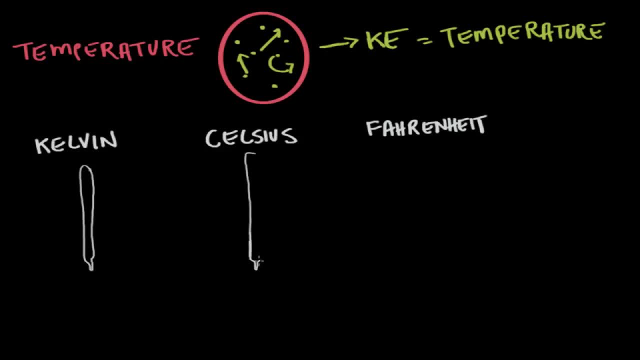 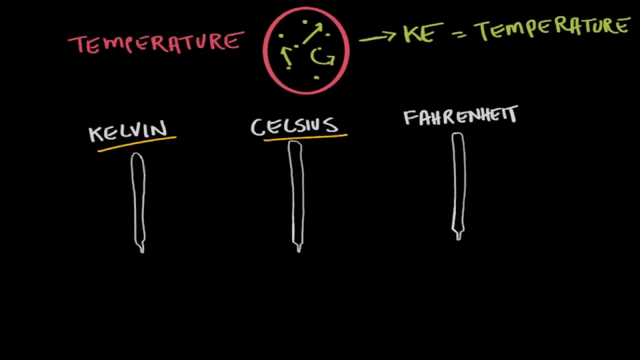 So one for Kelvin, and then we have a thermometer for Celsius and then another thermometer for the Fahrenheit scale, And the two scales used most in the physical sciences are probably the Celsius scale and the Kelvin scale. So as a point of comparison here on these thermometers, the freezing point of water, 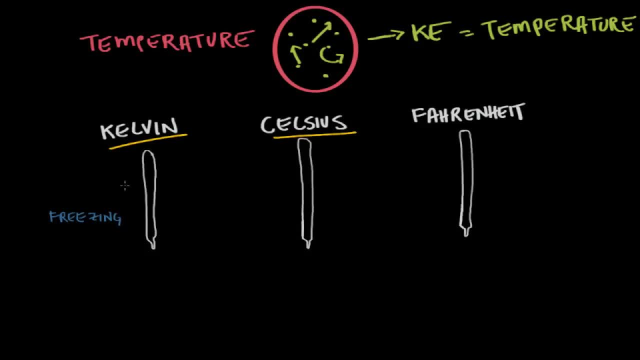 occurs at zero degrees Celsius. So we have zero degrees Celsius. That's where water freezes. And then the boiling point of water occurs at 100 degrees Celsius. So the boiling point of water occurs at 100 degrees Celsius. That's where water turns into steam, And I'm going to write H2O here real quick. 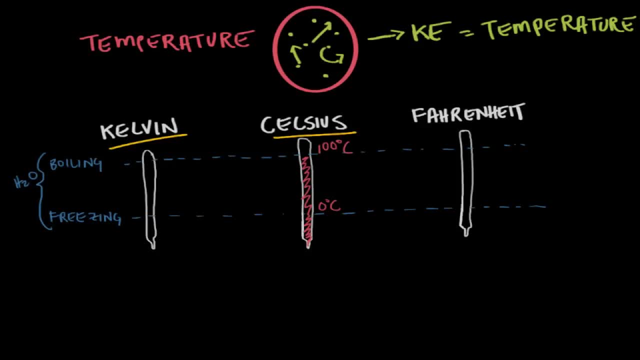 just so we don't get confused that we're talking about the freezing and boiling point of water. Now, when we use the Kelvin scale, we find that water's freezing point is 273.15 Kelvin And then we find that water boils at 373.15 Kelvin. 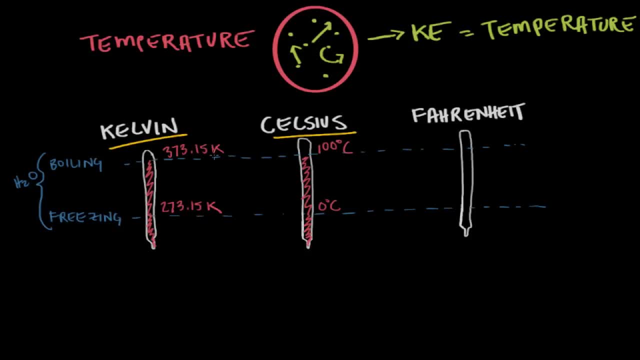 So they differ fundamentally in the zero point. The Celsius and Kelvin scales differ in the zero points that they use. But between water's freezing point and water's boiling point we have a span of 110 degrees Celsius, And then we have the freezing point, And then 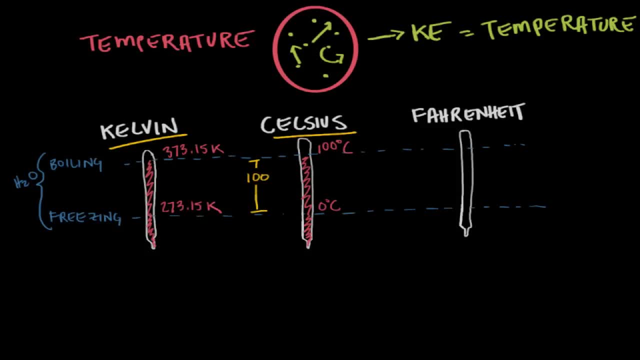 we have the freezing point, And then we have the boiling point, And then we have the freezing point, temperature units for both scales. So, although they differ in the zero points that they use, they use the same size unit or the same magnitude of unit to measure the temperature, So converting 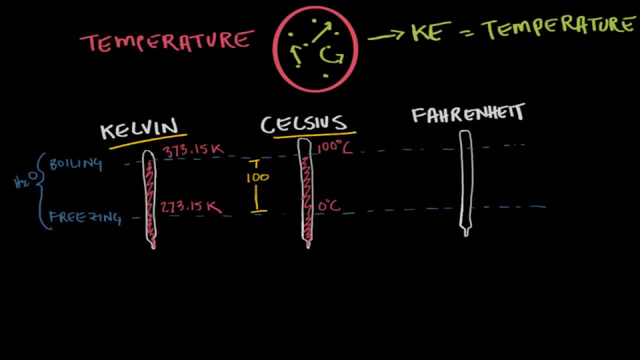 then between the two scales only really requires that we make an adjustment for the two different zero points. And this is what I mean. If we want to know the temperature in Kelvin, all we need to do is take the temperature in Celsius and add 273.15 degree units to it. So if we want to know, 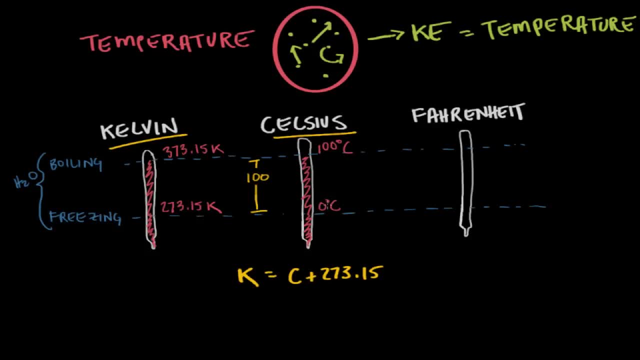 the temperature in Kelvin for the freezing point of water. we take the temperature in Celsius, which would be zero, and we add 273.15 units to it, and that would give us 273.15 Kelvin. Now if we want to flip that and if we want to find the temperature in Celsius from Kelvin, all we have to do is take: 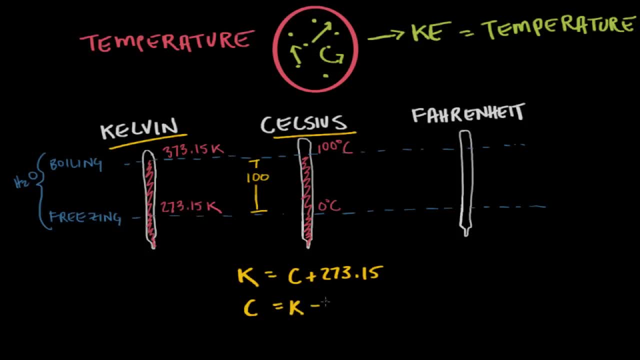 the temperature in Celsius and add 273.15 units to it, And that would give us 273.15 Kelvin. And so we would see that 373.15 Kelvin minus 273.15 would give us 100 degrees Celsius. So, just as 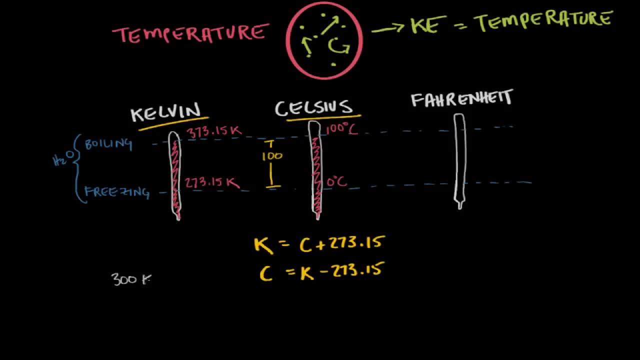 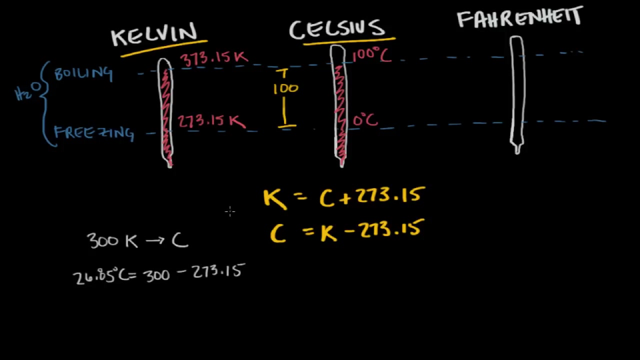 another example: let's convert 300 Kelvin to Celsius And, to start, since we're looking for the temperature in Celsius, we'll subtract 273.15 from it And that's going to give us 26.85 degrees Celsius. So 26.85 degrees Celsius is the same thing as 300 Kelvin, And I just want to point out really. 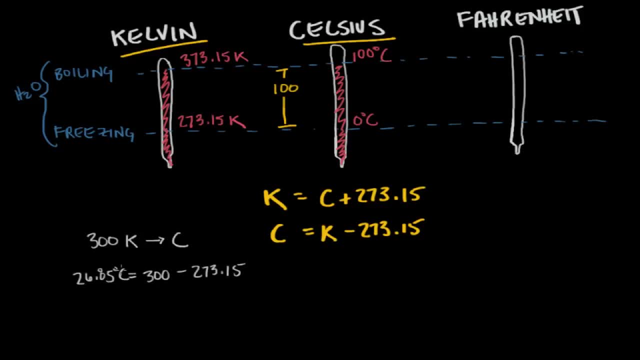 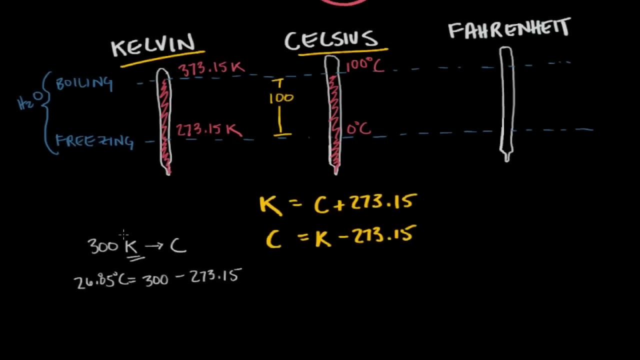 quickly that I'm only using the degree symbol here for Celsius, And I'm doing that intentionally. We don't need this symbol with Kelvin scale, because instead of calling the temperature units degrees, we just call them Kelvin. So the only thing we need is an uppercase K. Now converting between the 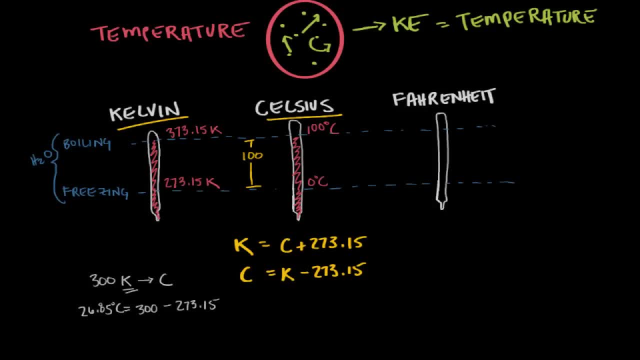 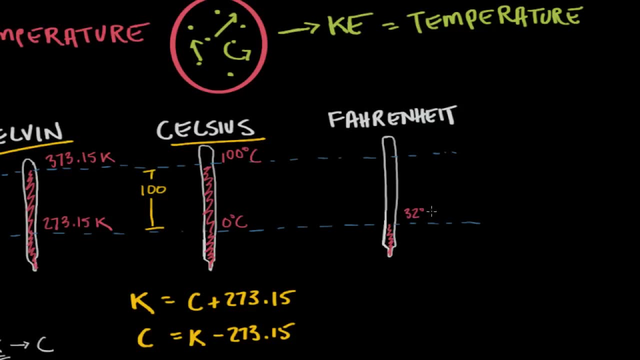 Celsius and Fahrenheit scales is a little bit more complicated. You see, in Fahrenheit water freezes at 32 degrees Fahrenheit, So 32 degrees Fahrenheit, And water boils at 212 degrees Fahrenheit, So 212.. And this gives us a span between the freezing point and the boiling point of water of a. 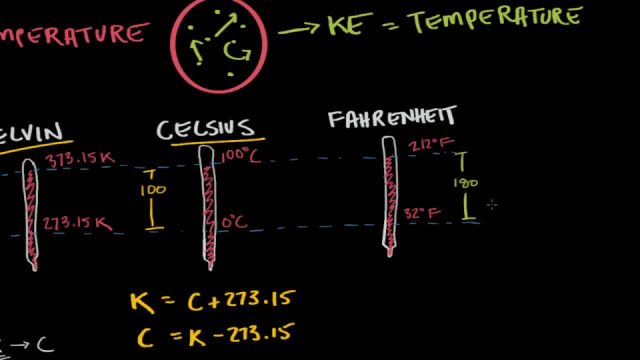 180 degree units. So we're going to need to consider two different adjustments here: One for degree size, because the units have a different magnitude: The same value or the same span of temperature is 100 units in Celsius and 180 units in Fahrenheit. And we're also going to need to 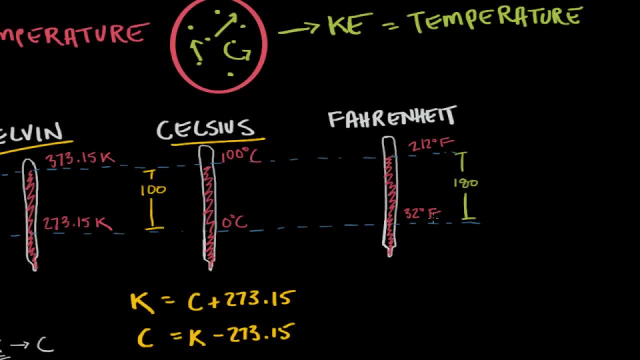 account for the two different zero points: Zero degrees Celsius for freezing and 32 degrees Fahrenheit for the freezing point of water. So first we can say that 180 degrees Fahrenheit is equal to 100 degrees Celsius, And again we can say this because both of these magnitudes refer to. 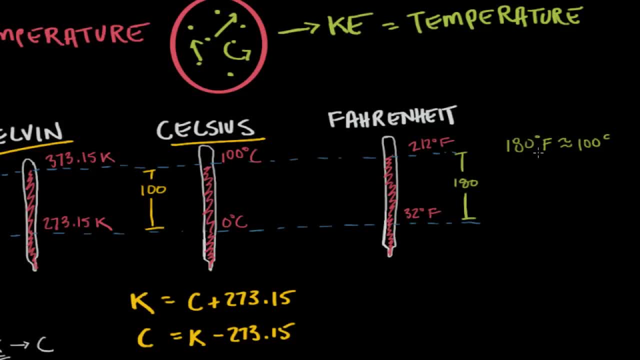 the same change in total energy. And so if we write this as a ratio, we have 180 over 100, which just reduces down to 9 over 5.. So the ratio of Fahrenheit to Celsius is 9 to 5.. Now we need to think about: 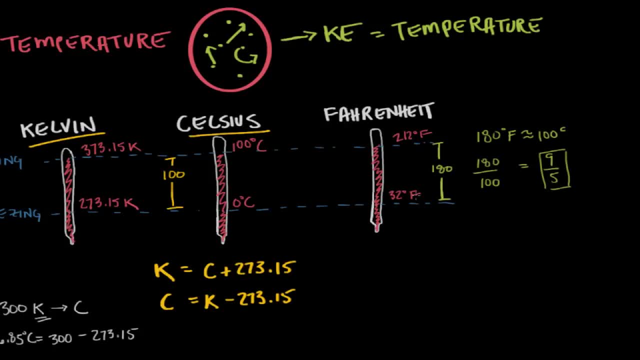 the two different ratios. So we have 180 degrees Celsius for freezing and 32 degrees Fahrenheit, And because 32 degrees Fahrenheit is equal to 0 degrees Celsius, we can find the Celsius temperature if we take the temperature in Fahrenheit and we subtract 32 degrees from it, And this makes sense. 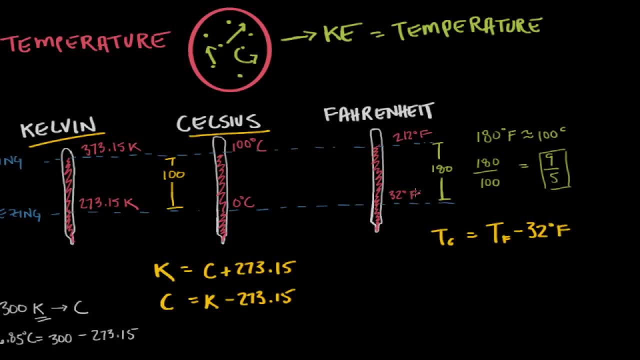 because 32 degrees Fahrenheit minus 32 degrees Fahrenheit would give us 0 degrees Celsius, And now we just need to apply the unit ratio. So, just like any dimensional analysis problem, we need to cancel out the degrees of temperature, And so we're going to need to cancel out the degrees of. 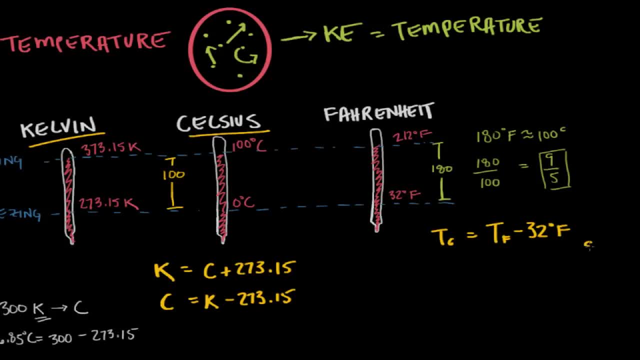 Fahrenheit. So if we put the degrees Fahrenheit on the bottom here- so 9 degrees Fahrenheit- we can cancel out the Fahrenheit, leaving us with just degrees Celsius. So to find the temperature in Celsius we take the temperature in Fahrenheit, subtract 32 from it and multiply it by a ratio. 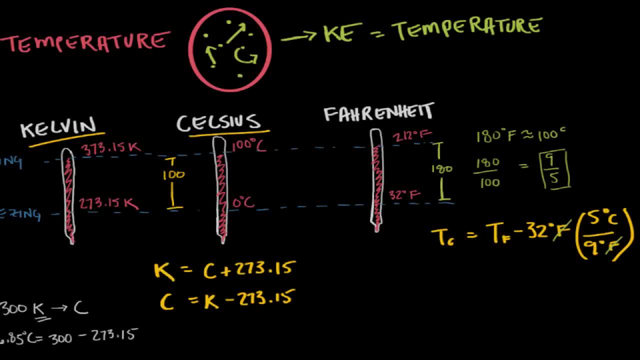 of 5 to 9.. And then we can also manipulate this formula if we want to start with Celsius, So all we have to do is solve for the the temperature in Fahrenheit, And so to start, we're going to need to divide both sides by 5 over 9.. Or that's the same thing as multiplying by the reciprocal. So, and then 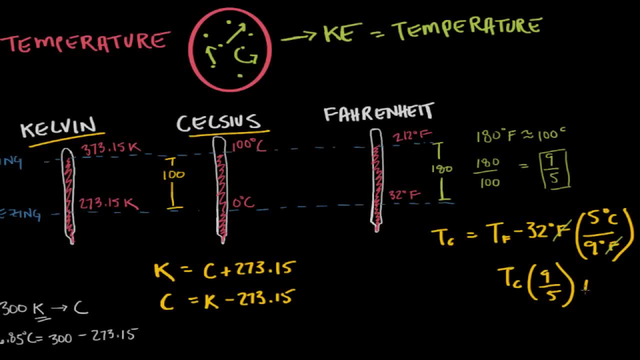 to finish it off, we would just add 32.. So plus 32 is equal to the temperature in Fahrenheit. So now, if we want to start with temperature in Celsius, we can move to temperature in Fahrenheit. Or we could start with temperature in Fahrenheit and move to temperature in Celsius, And so: 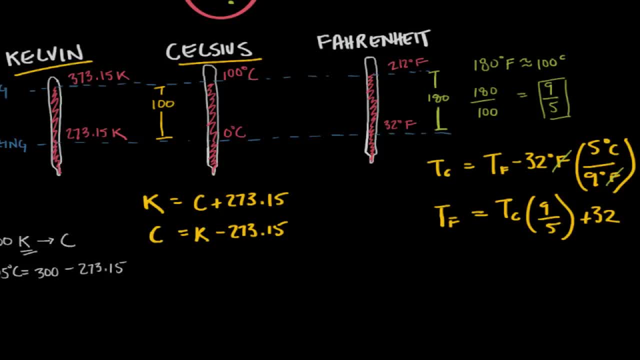 to practice this, let's go from Celsius to Fahrenheit, And it turns out that these temperature scales actually cross paths at a temperature which is kind of a kind of a fun fact. So if we plug in negative 40, let's go from negative 40 degrees Celsius to Fahrenheit. 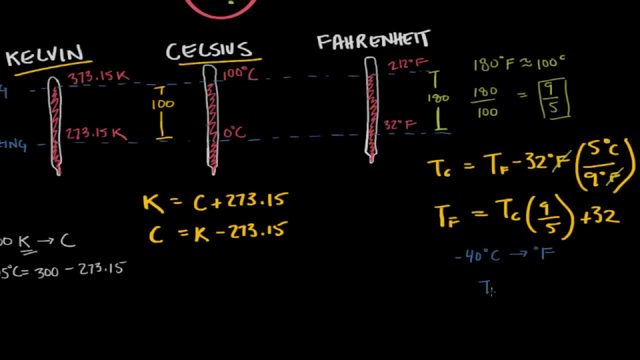 We'll find that Tf is equal to negative 40 times 9 fifths plus 32.. And so we can reduce this term here. so 5 and negative 8, or 5 and negative 40 reduces to negative 8.. So negative 8 times 9 plus 32.. 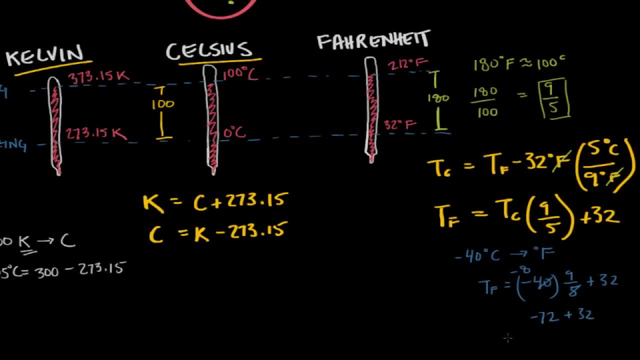 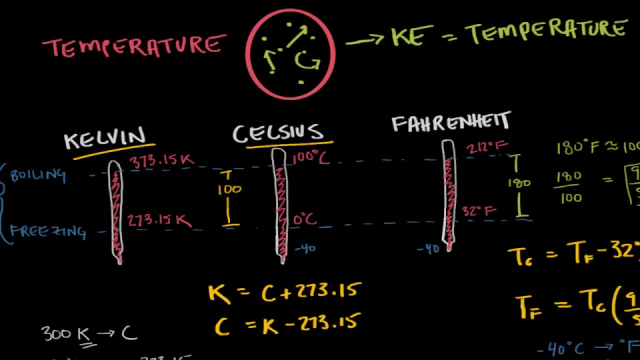 That's negative 72 plus 32. So the temperature in Fahrenheit would equal negative 40 as well. So negative 40 degrees Celsius is the same thing as saying negative 40 degrees Fahrenheit. That's kind of just a fun fact. And another observation from this little factoid is that Celsius and Fahrenheit scales can both have negative or positive values. 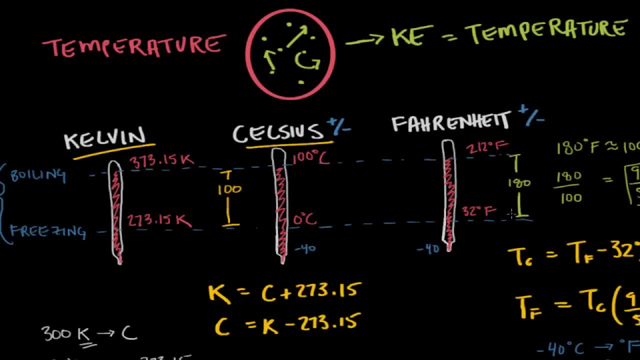 We see that both can be negative 40. So these can both have negative values, And that's actually a point where they differ from the Kelvin scale. The Kelvin scale can only have a positive value And it turns out that the absolute coldest temperature is 0 Kelvin. 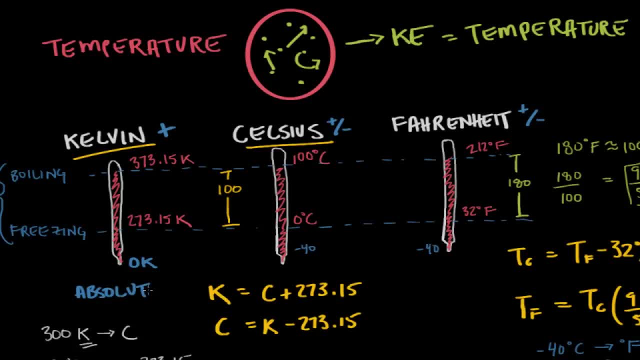 So 0 Kelvin is absolute, Absolute, absolute 0.. And the reason we can't get any colder is that at this point no particles would have any kinetic energy, And so that means no motion at all. We said that temperature is a measure of the kinetic energy. 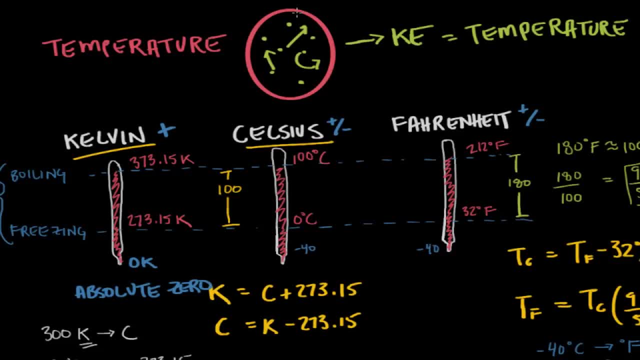 And the coldest that you can get is no kinetic energy whatsoever. And it turns out that the laws of physics, specifically the uncertainty principle, just don't allow for this. So we can get close, like within a billionth of a Kelvin, but we can't get all the way there. 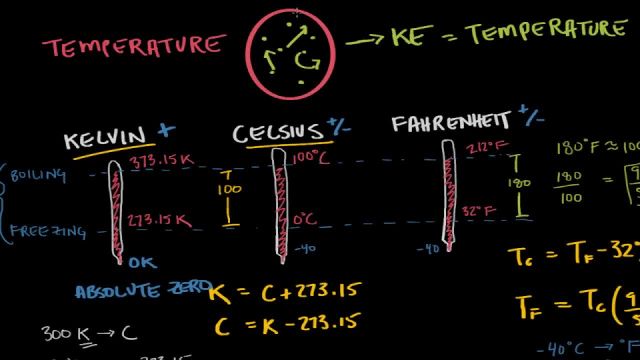 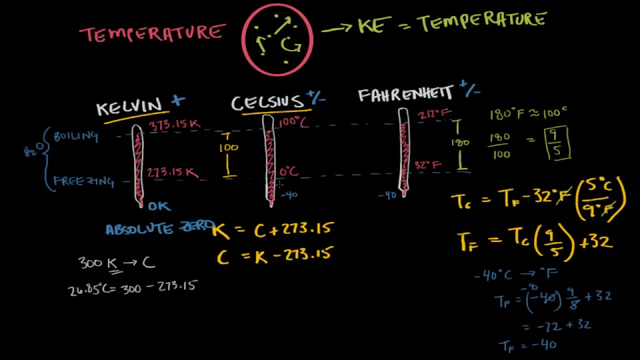 And because Kelvin scales Always has a positive value, it becomes a little handier in various formulas And so it's used as the standard, the SI unit for temperature. So I'll show you in future videos why absolute 0 happens at negative 273.15 degrees Celsius.